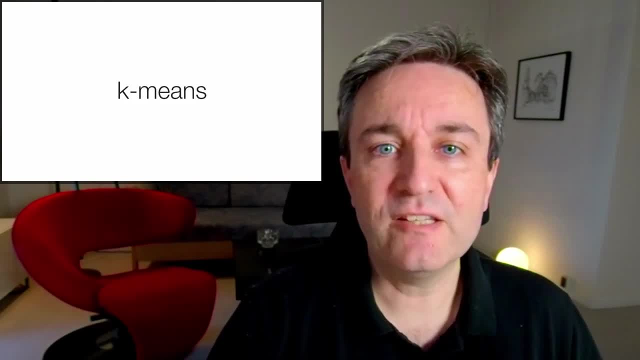 There are several algorithms for this. the best known is probably the k-means algorithm, in which in the original input coordinates and try to define centroids that correspond to the clusters. Another popular clustering algorithm is Markov clustering, also called MCL, which takes the network view on the data and tries to do community detection. 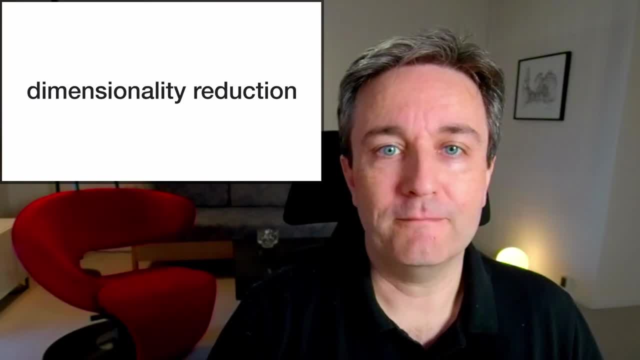 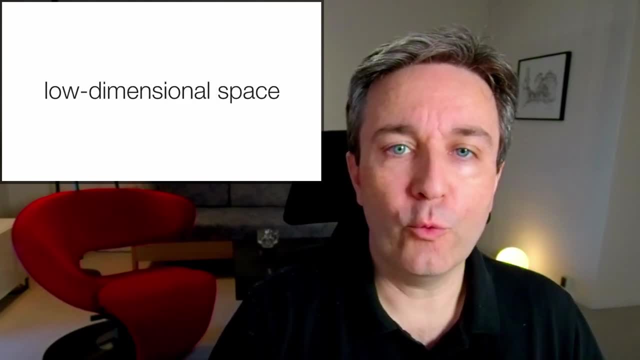 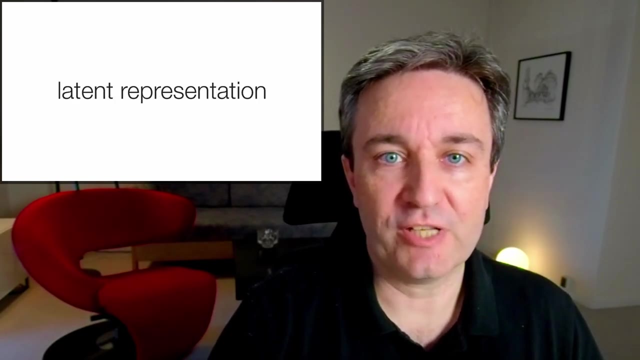 Another class of unsupervised learning is dimensionality reduction. The goal here is very different, namely to take the high dimensional input data and compress it to produce a lower dimensional space that captures the information. This lower dimensional space is also called a latent representation of the input data. 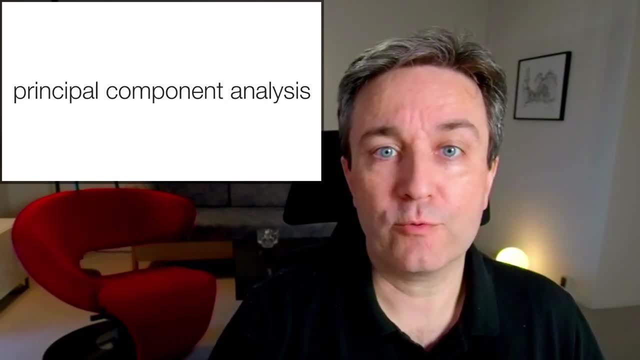 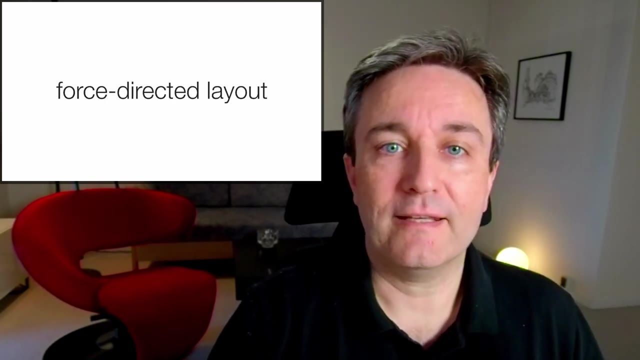 There are several methods. some are linear, the best known being, of course, principal component analysis, and most of them are non-linear, including TISNI and UMAP, both of which are commonly used for visualizing single cell data and also multi-dimensional scaling and force directed layouts. 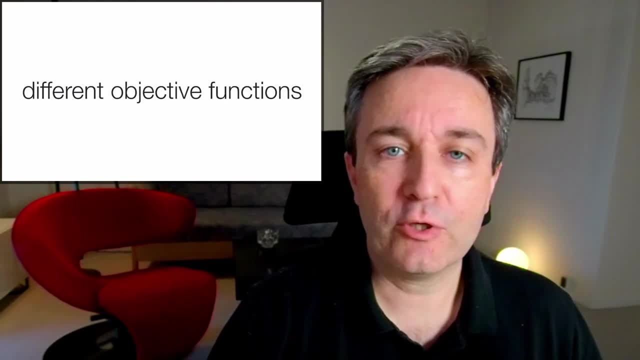 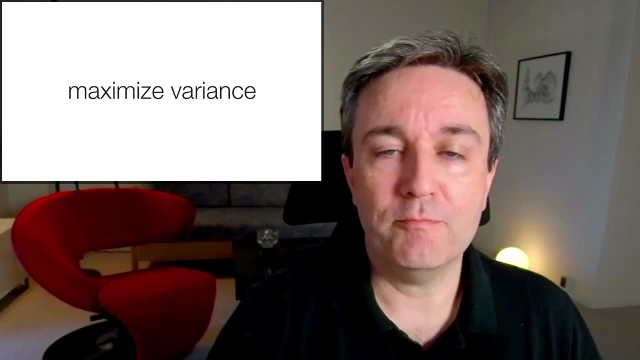 All of these algorithms do similar things, but they have different objective functions that are being optimized and different transformations that are allowed. For example, in PCA we try to maximize the variance captured in TISNI. we're focusing mainly on preserving the local structure. 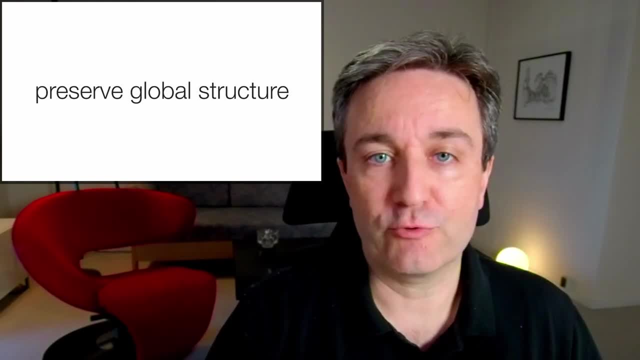 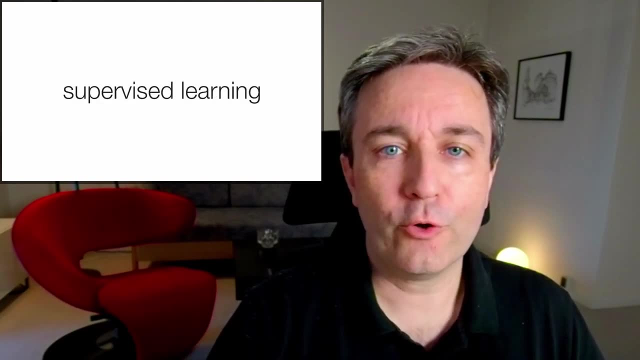 and UMAP tries to preserve both the local and the global structure. Another approach to dimensionality reduction is autoencoders. Autoencoders are, in a way, supervised learning, But instead of trying to learn to predict the output from the input, it tries to predict the input from the input. 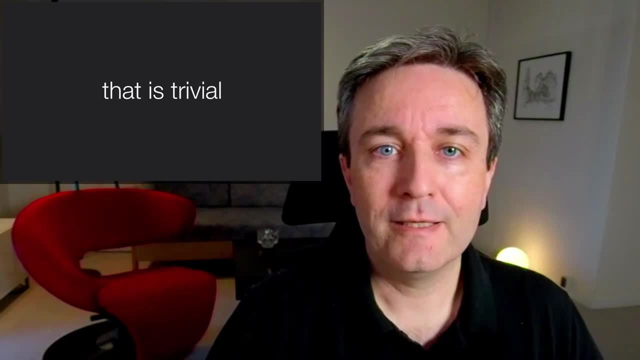 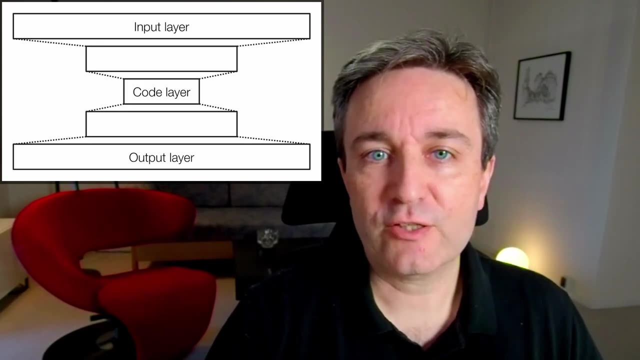 You might, of course, object that's trivial and that's true. But what we do is we introduce a bottleneck in the neural network architecture. So we work with an architecture that looks like this, where you have an input layer, then possibly a hidden layer with lower dimensionality. 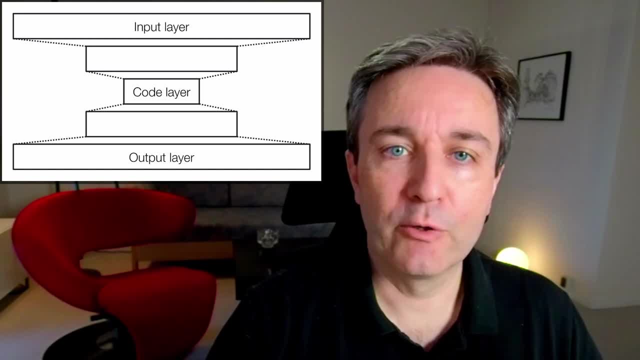 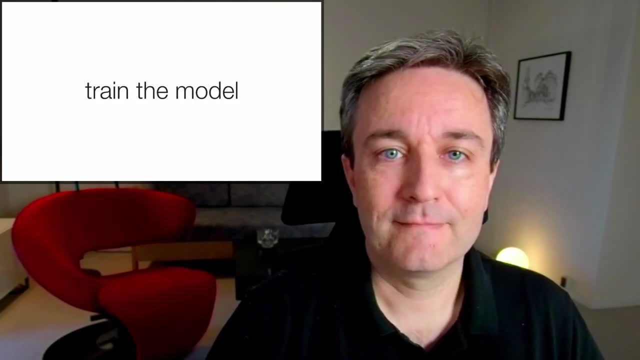 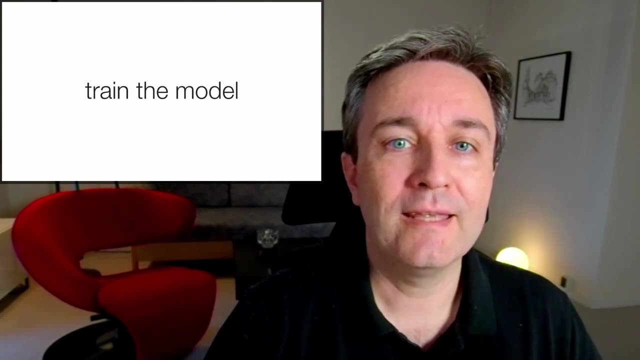 the small code layer in the middle and then mirroring the architecture in the other half to again produce an output layer with the same size as the input layer. The trick here is that when we train the model, it has to learn in the code layer a low dimensional representation of the data that allows the high dimensional version to be reproduced faithfully. 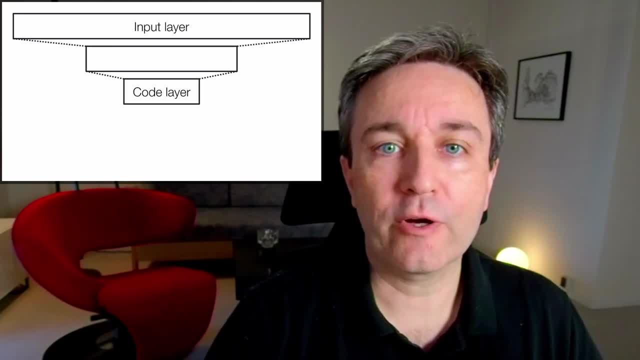 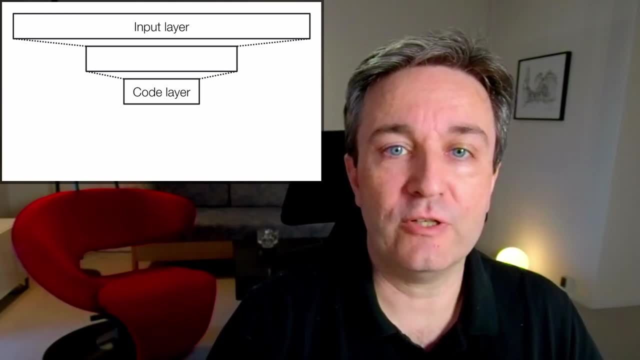 After having trained it, we can throw away the lower half of the network and now have our autoencoder that takes the data in the input layer and converts it into a low dimensional representation in the code layer, in other words, the latent representation. 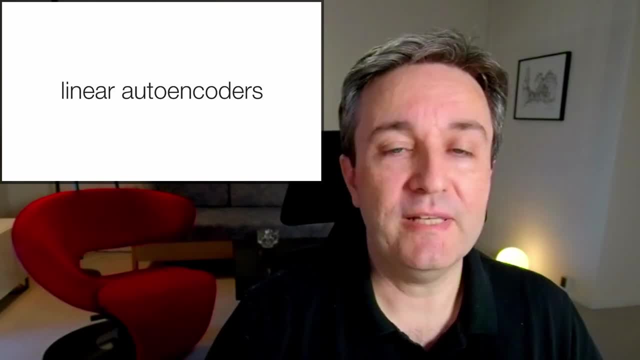 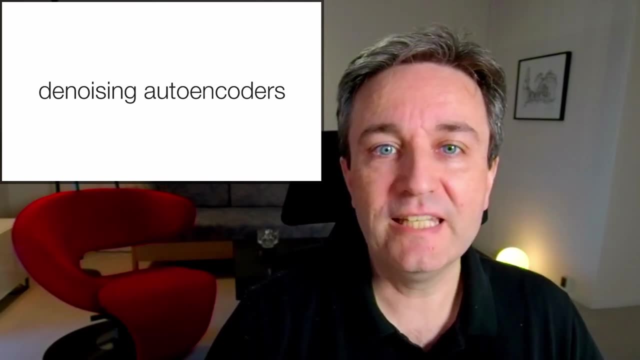 There are many variants of autoencoders. Autoencoders can be linear, but most autoencoders are non-linear. In addition to normal autoencoders, you have denoising autoencoders that take a noisy version of the input data and tries to reproduce the clean version of the input data. 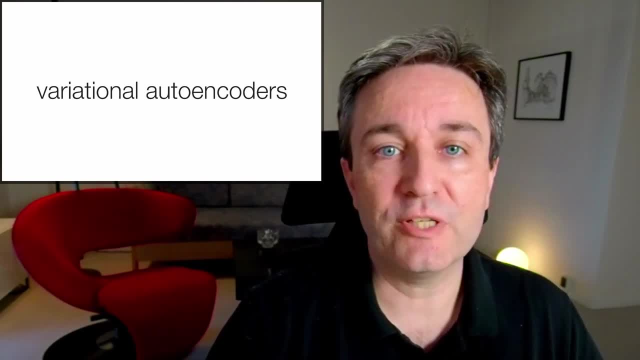 And you have variational autoencoders that have become very popular recently that in turn, are more generic, and you have variational autoencoders that have become very popular recently that, in turn, are more generic. instead of learning a single vector representation in the middle, rather learn a Bayesian representation. 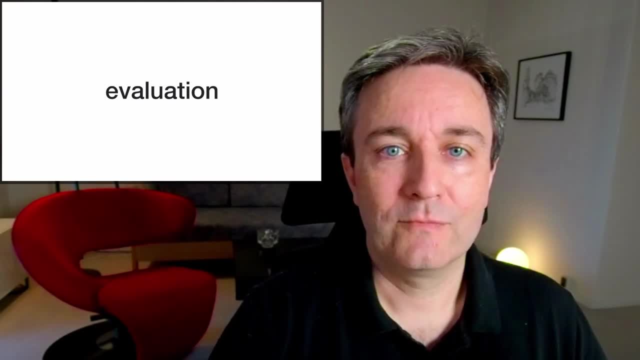 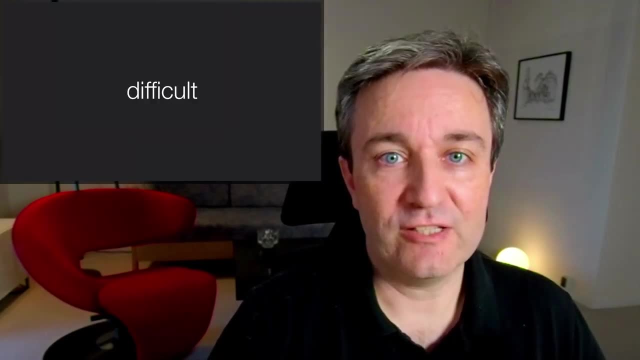 of the data. So let's say we've done some unsupervised learning. How can we evaluate the quality of the results? The short answer is: it's difficult, And the reason is that we don't know the ground truth. That's why we're doing unsupervised learning. 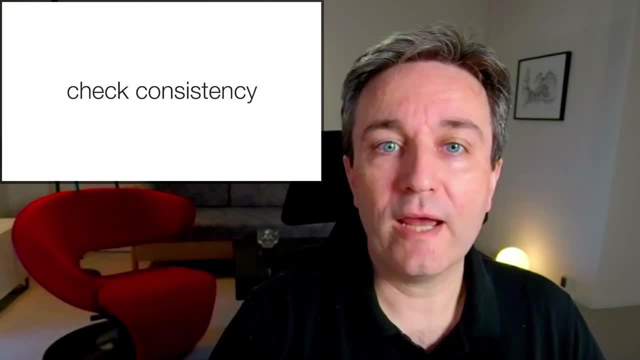 If you have some labels for some of your data points, it's very wise to check for consistency, In other words, whether the structure you found in the data is consistent with what you know about your data points. Alternatively, if you're doing clustering, you can use metrics like intra-cluster cohesion. 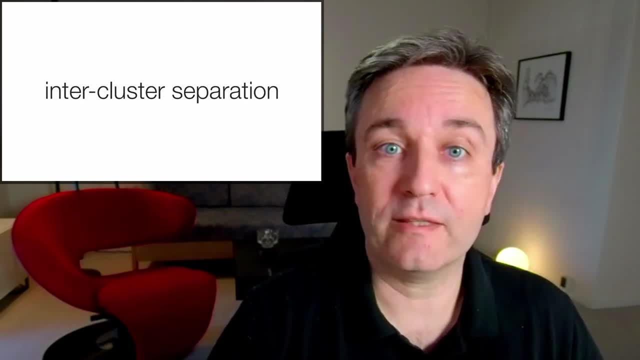 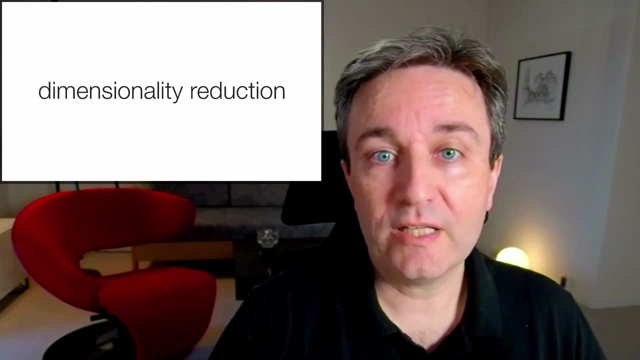 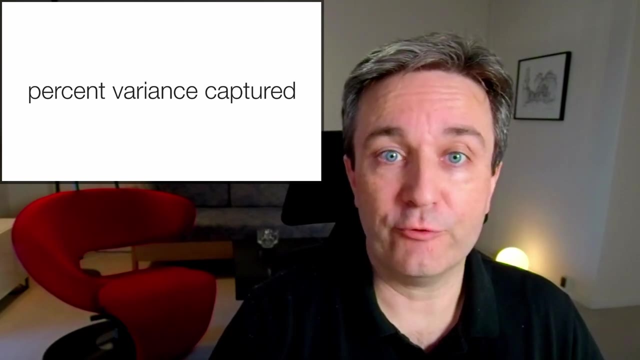 and inter-cluster separation, In other words, looking at whether the points within clusters are indeed much closer to each other than the points in different clusters. If you're doing dimensionality reduction, for example PCA, you will want to look at how much of the variance do you manage to capture in the first few dimensions. 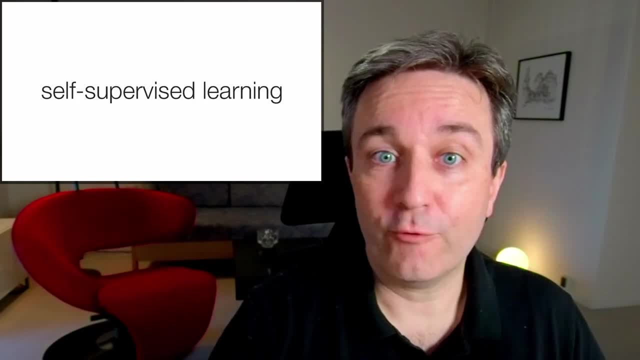 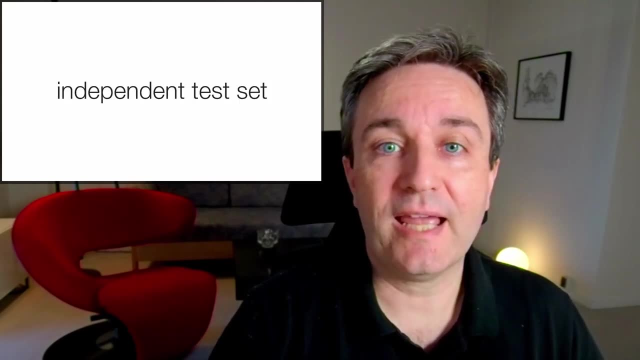 And if you're doing autoencoders, which are a form of self-supervised learning, you can of course steal the tricks from supervised learning, leave out some of the data and thereby have an independent test set to see if your autoencoder indeed works also on new data. 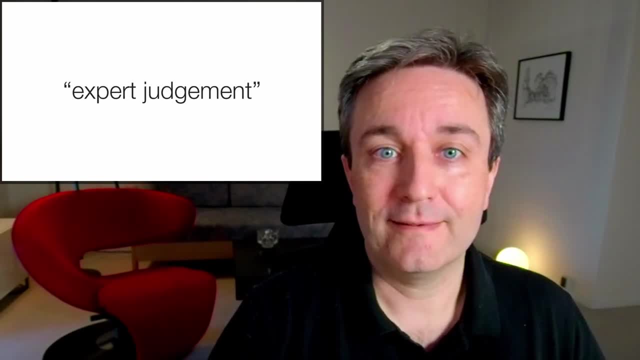 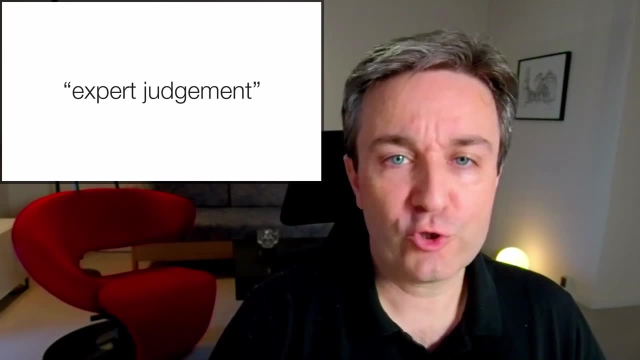 But in the end it typically comes down to expert judgment. That is, having somebody who knows about the data. look at your unsupervised learning and see if it makes sense. Alternatively, something that I like to do, It's what I call downstream benchmarking.